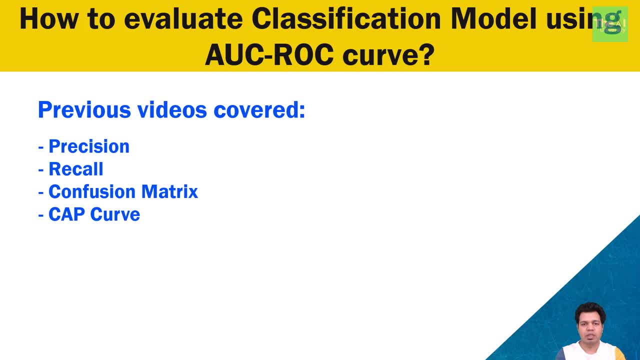 In the previous video I covered various other classification model evaluation techniques like precision, recall, confusion matrix, as well as cap curve. Here I will cover AUC ROC curve. So what exactly is AUC ROC curve? Well, AUC ROC curve is a classification model performance measurement metric which tells us 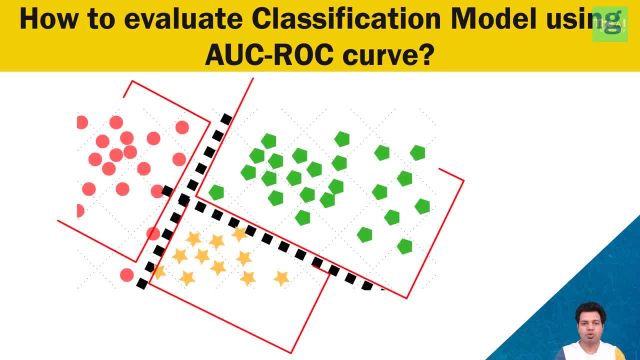 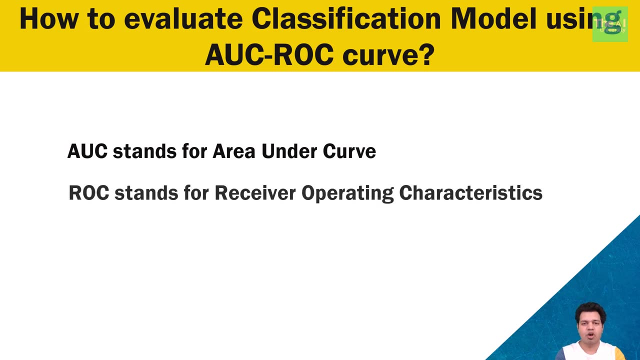 how much a classification model is capable of distinguish between the classes. Using AUC ROC clock can continue to visualize the performance of a multi class classification problem as well. So we have AUC stands for area of a city under the curve and ROC stands for receiver of operating. 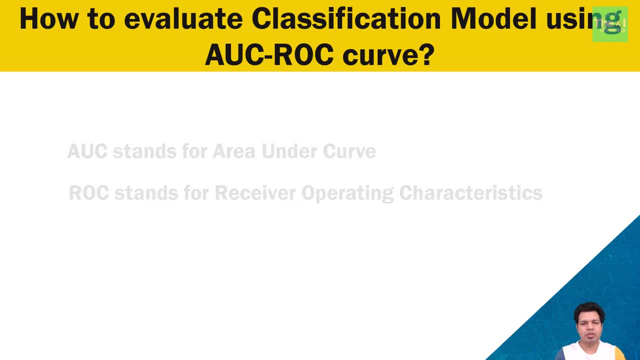 characteristics In AUC ROC curve. AUC represents the degree or measurement for separability and ROC represents probability curve. So if the querer is higher, then it means that the model is better at predict classes. model is quite good at predicting spam as spam and not spam as not spam. Please note that we. 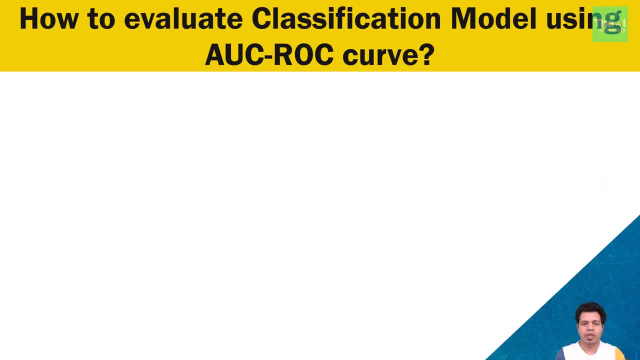 should be aware of certain concepts before we jump on to AUC ROC curve, and these concepts are: confusion matrix, true positive rate, false positive rate, recall, sensitivity, specificity, etc. Please note that true positive rate or recall or sensitive is one and same thing. So if someone 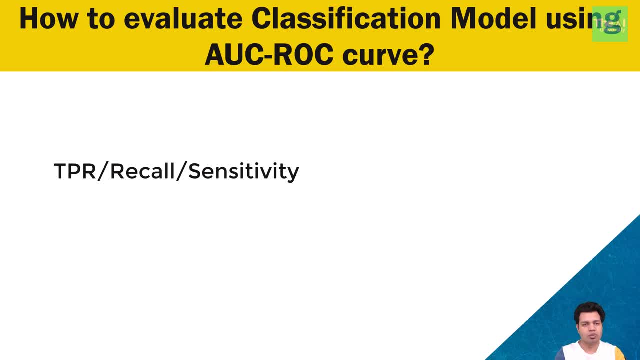 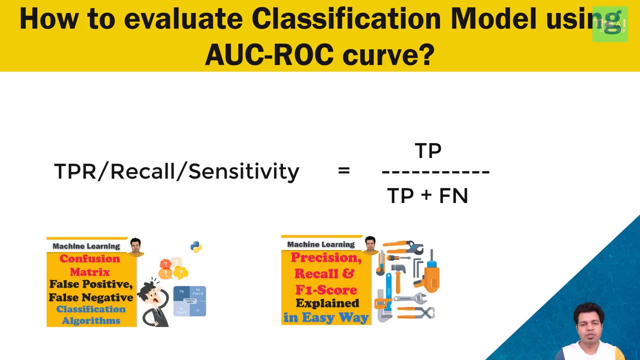 is saying recall, then it means that he is talking about true positive rate or sensitivity. The formula of these three terms is same and it is true positive divided by true positive plus false negative. I have already created a video on confusion, matrix, precision and recall, so you can. 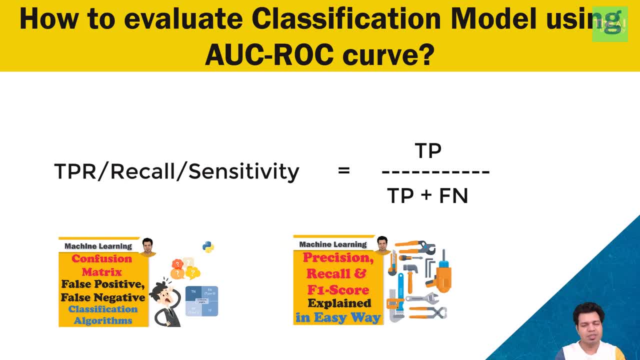 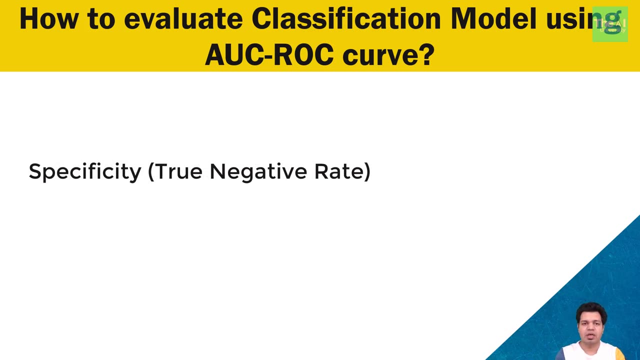 watch that video to a quick acquire the necessary knowledge. In this video I am going to cover false positive rate and specificity before moving ahead with AUC ROC curve. So let me first explain specificity. Specificity, which is also known as the true negative rate, measures the proportion of actual 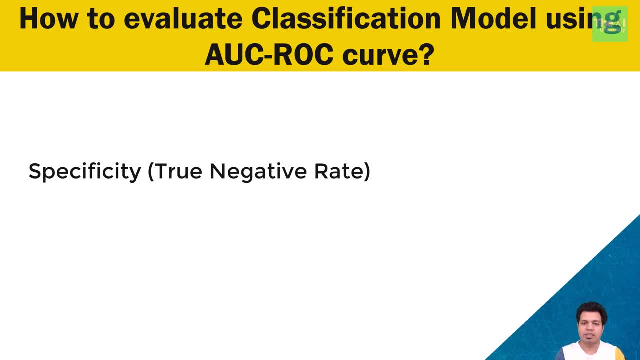 negatives that are correctly identified. as such, The formula of specificity is true- negative divided by true- negative plus false- positive. So specificity tells how good our model is at identifying the false or negatives correctly. Please note that sensitivity and specificity are inversely proportional to each other. Therefore, when we increase sensitivity, 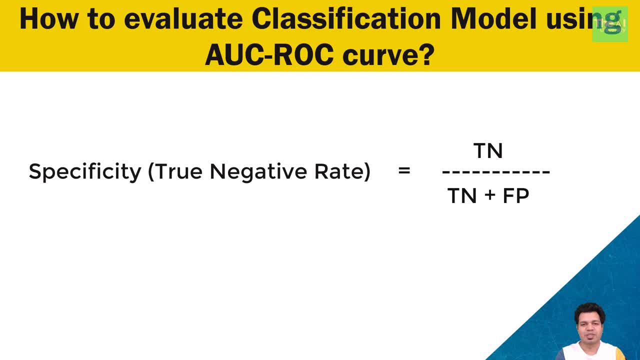 specificity decreases and vice versa. You also need to remember that when we decrease the threshold, we get more positive values, hence it increases the sensitivity and decreasing the specificity. Similarly, if we increase the threshold, we get more negative values Done, we get higher specificity and lower sensitivity, Moving on to false positive rate or F 돼요, which is: 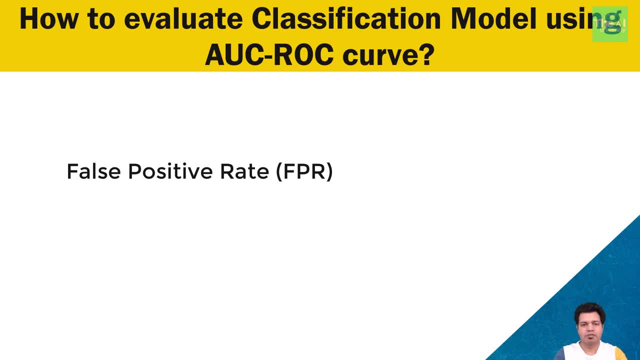 calculated as the ratio between the number of negative instances which are wrongly categorised as positive, ie false positive, and the total number of actual negative instances. so here is the formula for the same. So false positive rate ist equal to false positive divided by false positive plus true negative. False positive rate tells us that 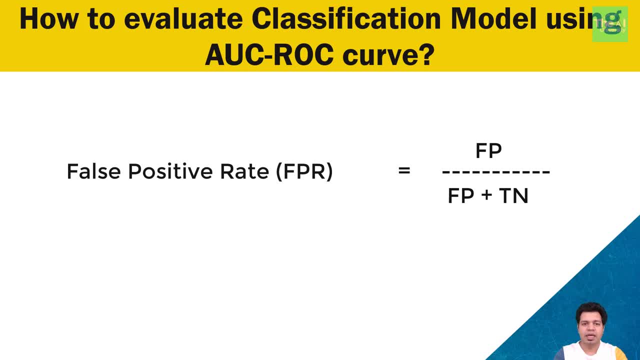 when the actual value is negative or false, then how wrongly have the classification model performed to classify the data? That is, if we look at only the negatives or false, then how wrongly the model has classified them as positive. False positive rate can also be calculated as 1 minus specificity. 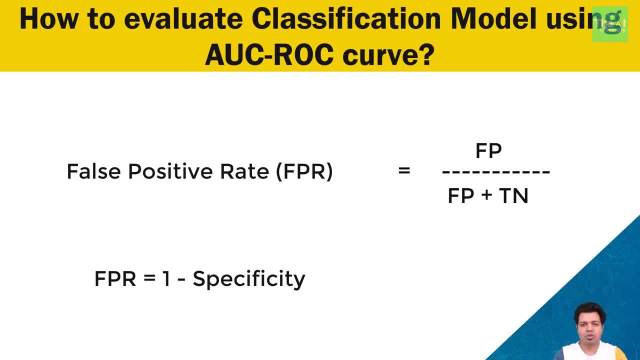 Let's move on to AUC ROC curve now. So the ROC curve is plotted with true positive rate against false positive rate, where true positive rate values are plotted on y-axis and false positive rate values are plotted on x-axis. So let me show you a plot first. So this is how the ROC curve. 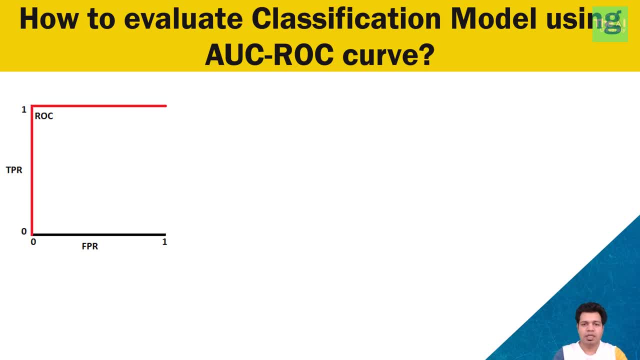 looks like True positive rate is on the y-axis and false positive rate is on the x-axis. ROC curve is the curve of probability, So the the corresponding distribution curves are represented like these: Here the area under curve is equals to 1.. So if our classification model is an excellent model, then it means that it has area under curve. 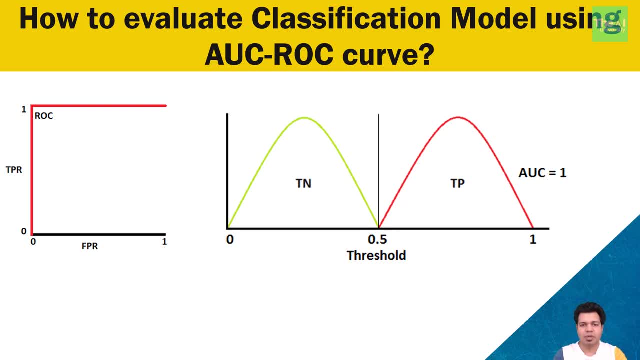 close to 1, which means it has good measure of separability. A poor model has AUC close to 0, which means it has worst measure of separability, which means that it is reciprocating the result, thereby predicting 0.. If the area under curve value is 0.5, then it means that model has no class separation capacity. 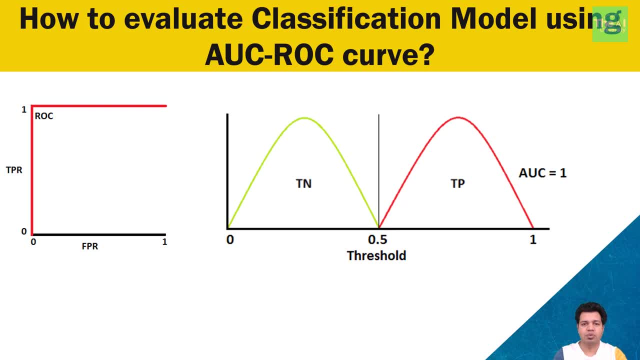 The plots shown here represents an ideal situation where two curves, that is, red and green curves, are not overlapping at all, Thereby suggesting that model has an ideal measure of separability. It is perfectly distinguishing between positive class and negative class, as you can see here, and here threshold is: 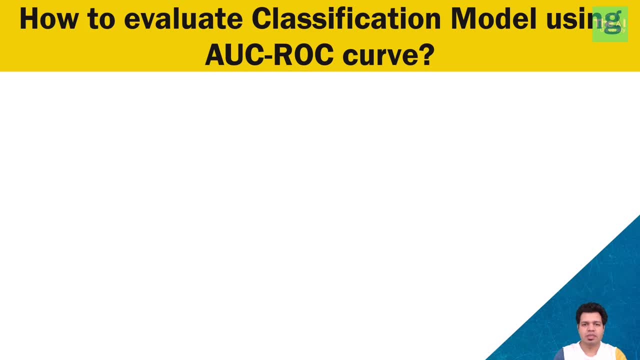 capped 0.5.. Now lets move onto another set of plots. We can see that ROC curve here is not ideal and area under curve in this case is less than 1.. and it is 0.7 here, which means that area under curve is less than what we had in the case of. 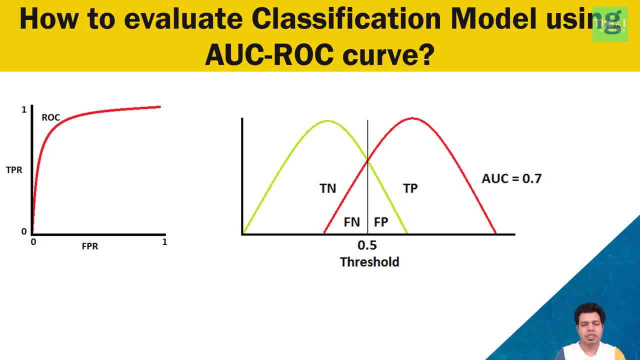 ideal ROC curve. This is because we have certain errors in the predictions or, in another words, there are certain instances where model is giving wrong predictions. So, Basically, there are certain type 1 and type 2 errors which got introduced in this model, due to which the area under curve is coming as 0.7.. 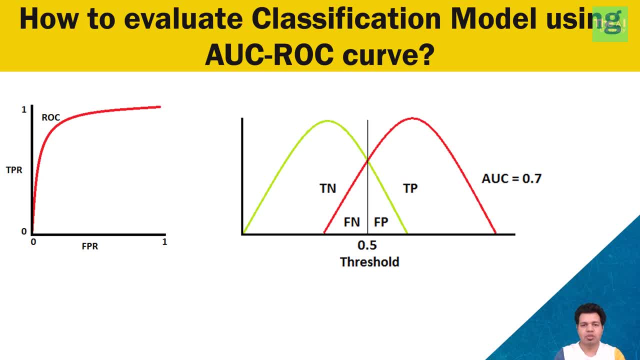 And if you don't know what are type 1 and type 2 errors, then you can watch this video. So here you could see that there is an overlap in two distribution curves, resulting in type 1 and type 2 errors. Now here, area under curve is 0.7, which means that there is a 70% chance that classification 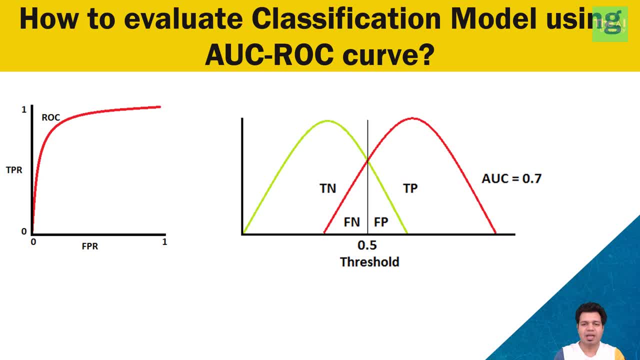 model will be able to distinguish between positive class and negative class. The area where this overlap is happening is shown as false positive and false negative. Threshold is again 0.5 here. Now let's consider another scenario, when AOC or area under curve is 0.5.. 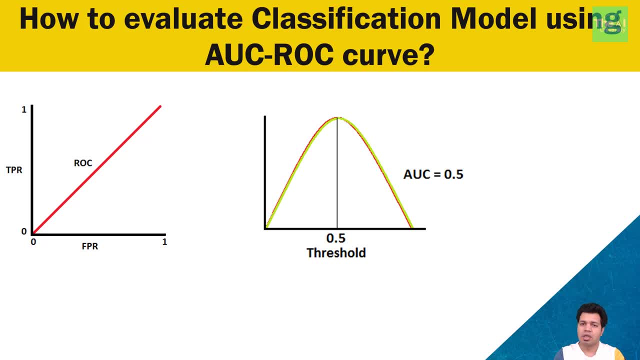 Here you can see that both of the distribution curves are 0.5.. Here you can see that both of the distribution curves are overlapping. ROC curve shown here is a random line in the middle. So this represents worst classification model, because this kind of model has no discrimination. 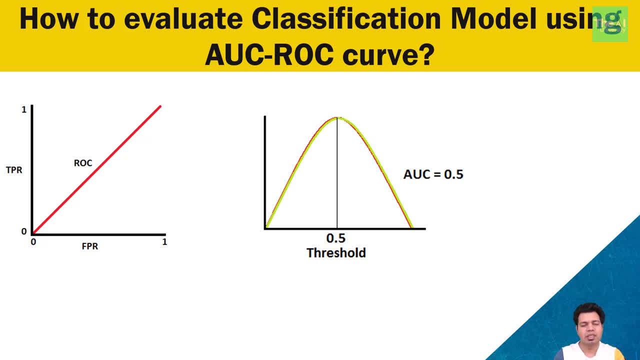 capacity to distinguish between positive class and negative class. Finally, let's consider another scenario: when AOC is equals to 0 or area under curve is equals to 0. So if you see, here there are two distribution curves where red curve, or true positive, has. 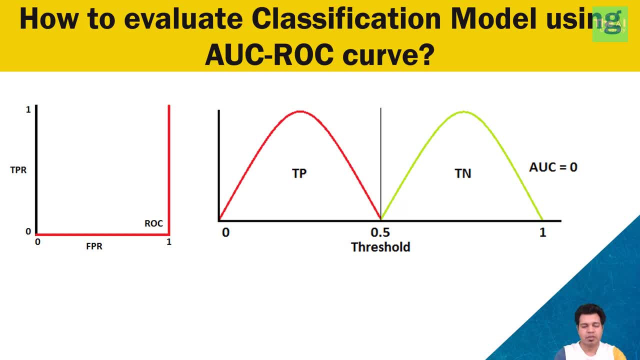 moved to left Left hand side and green curve, or true negative curve, has moved on to the right hand side. The ROC curve in this case is the reciprocal of ideal ROC curve, which was our first scenario. This represents the classification model which reciprocates the classes.